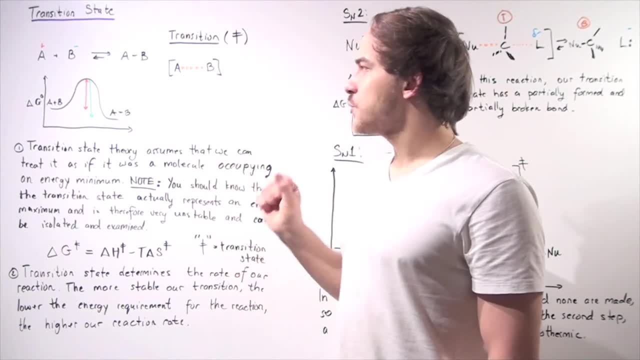 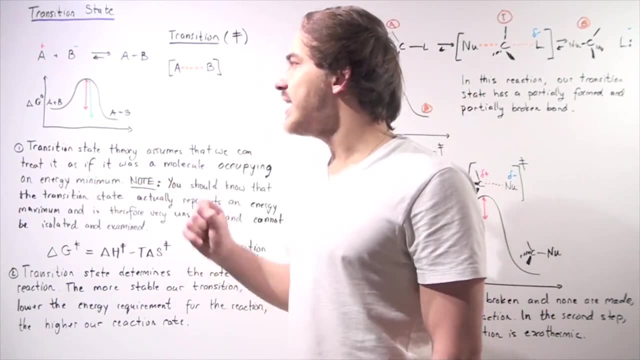 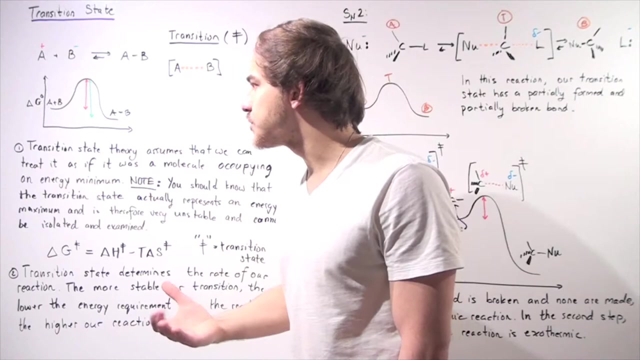 So let's describe the energy diagram for this reaction. Let's make the assumption that this is an exothermic exergonic reaction. So our y-axis is change in Gibbs, free energy on the standard state conditions, and our x-axis is reaction progress. 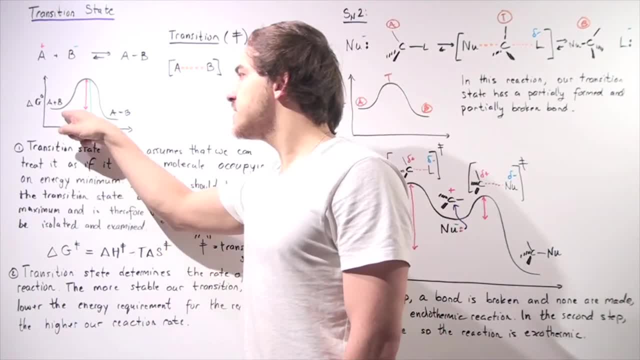 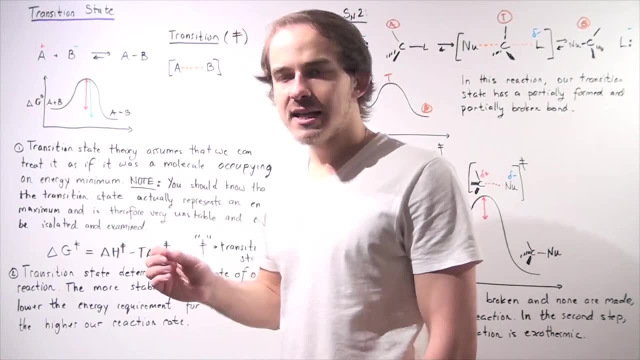 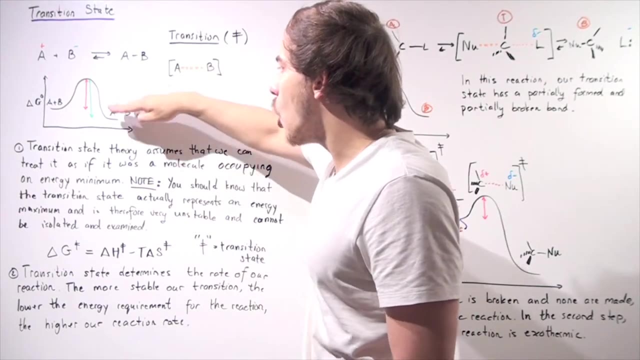 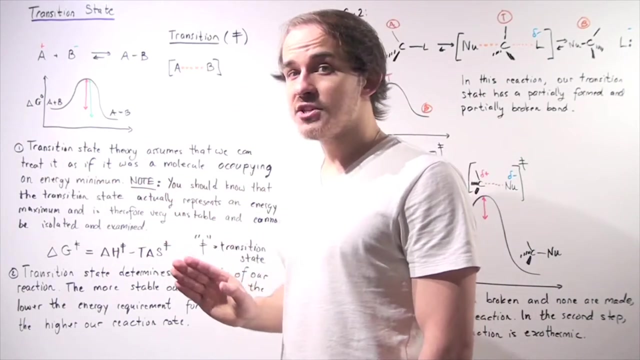 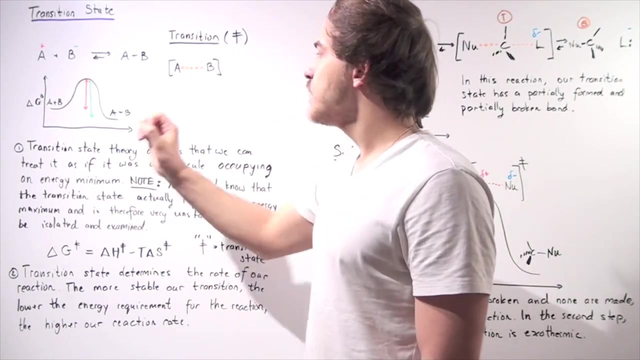 So let's suppose our reactants begin on this energy level, so A and B, And here we have our product. and because our reaction is exergonic, that means our change in Gibbs free energy is exergonic, And because our change in Gibbs free energy between our products and reactants will be negative, this will be lower in energy than our initial reactants. So we go from reactants in which we have no bonds between A and B to our product in which we have a fully formed covalent sigma bond between A and B. 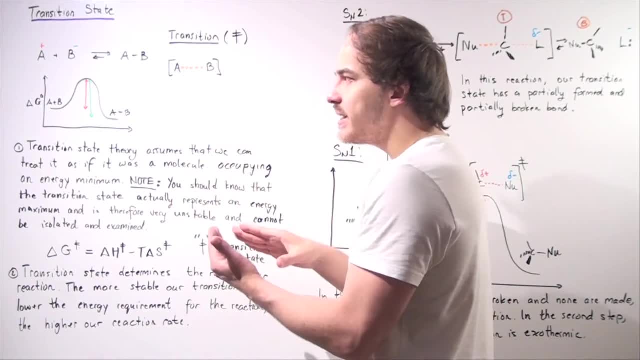 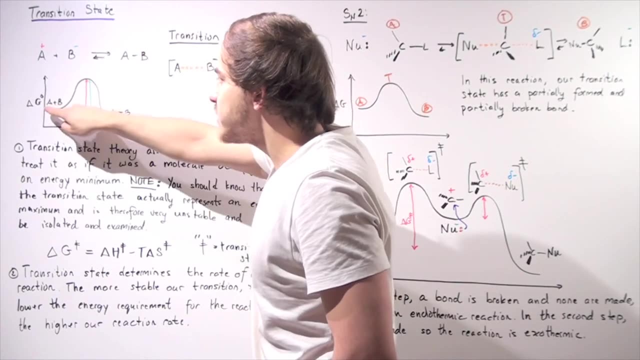 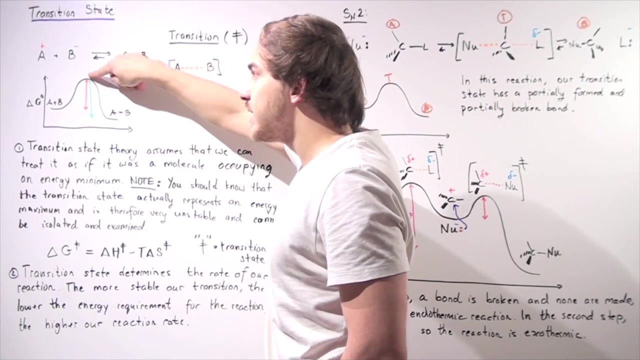 Now my question is: what's actually happening in between A and B? Well, in between A and B, is this energy maximization? Notice that this tip, on this mountain, on this energy curve, is the energy maximum. It's the highest point of energy on this diagram. 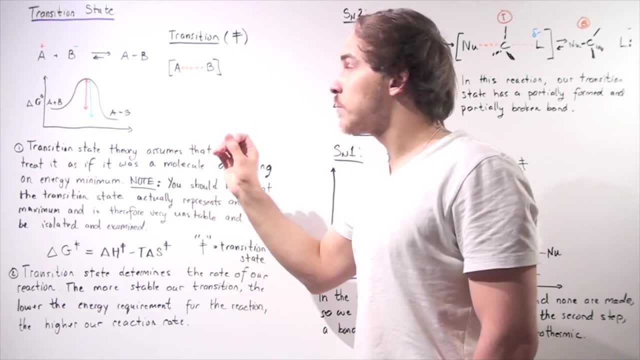 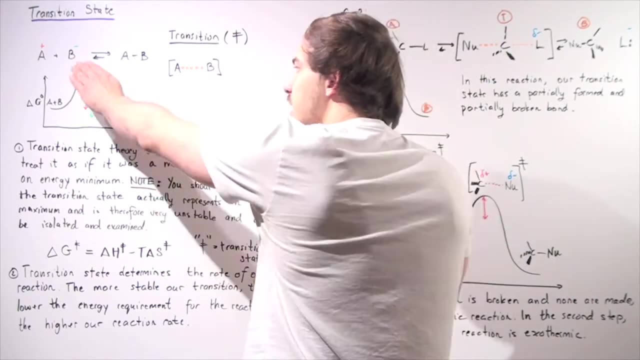 And this is known as our transition state, represented by this symbol here. So what's actually happening between our reactants A and B in the transition state? Well, if we go from no bond to a fully formed bond, that means in the transition state, in the milli находится, in which the reactants start to covalent. and if we go from li Bryant bond, we are in the transition state. 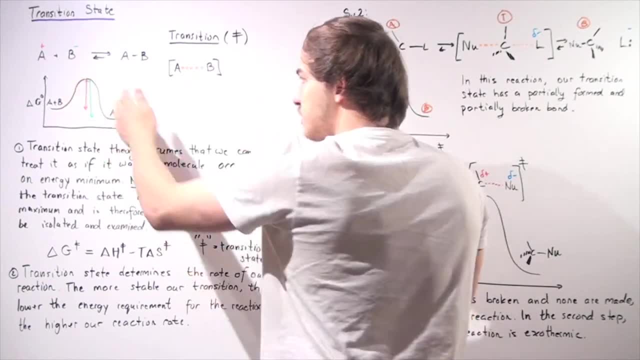 So usually the healing phase is from this first step of love. I'll just return after the transition. first step is l Netherlands bond and the next step is from no bond to a fully formed bond. that means in the transition state in the relay capacitor and and therefore the exchange of the energy. 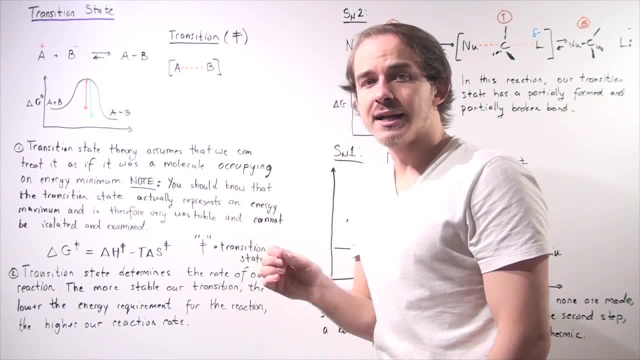 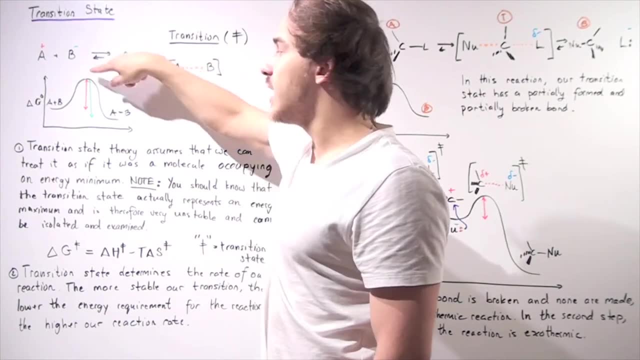 Let's look at another example here. let's dairy middle. we're going to have a partially formed bond. So this is what our transition state will look like on this energy maximum at this point on the curve. So we're going to have a partially 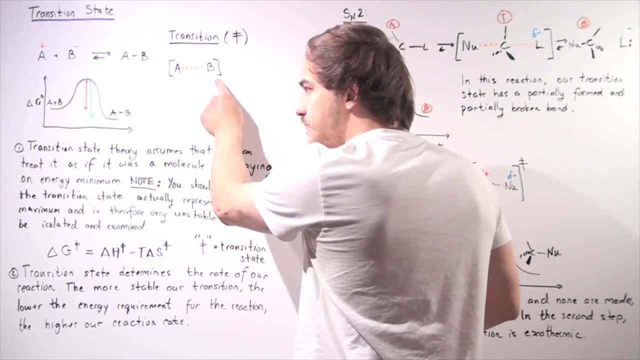 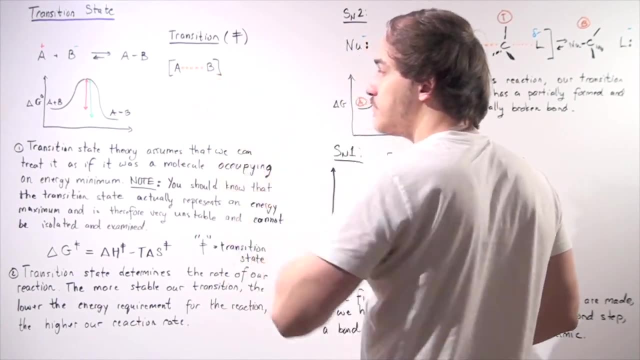 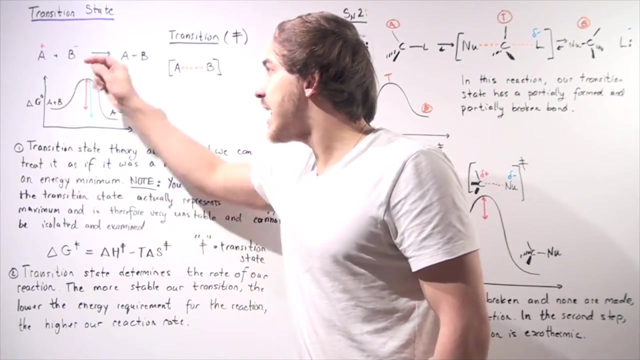 formed bond between A and B, So we're going to have a partially positive charge on A and a partial negative charge on B. Now notice that the transition state theory assumes that we can actually treat our transition state as if it was a molecule occupying an energy minimum. 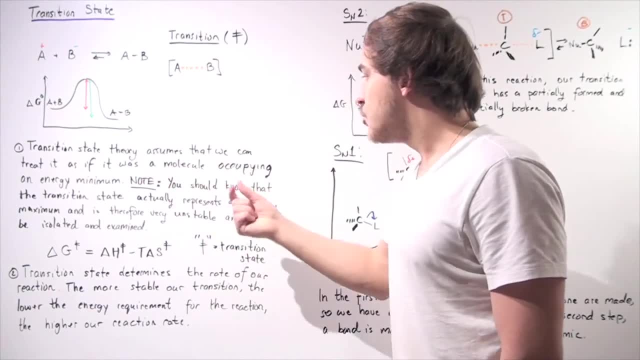 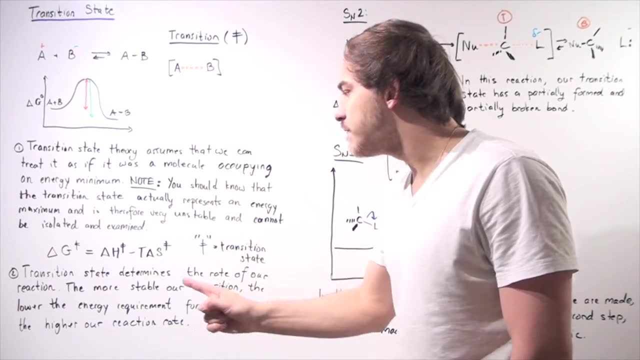 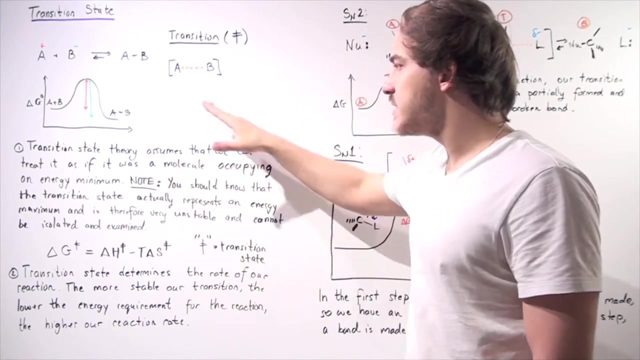 So, before we discuss this, let's read this note. Note: you should know that the transition state actually represents an energy maximum and is therefore very unstable and cannot be isolated. So let's begin by explaining what the second part of this state means. So, once again, this transition. 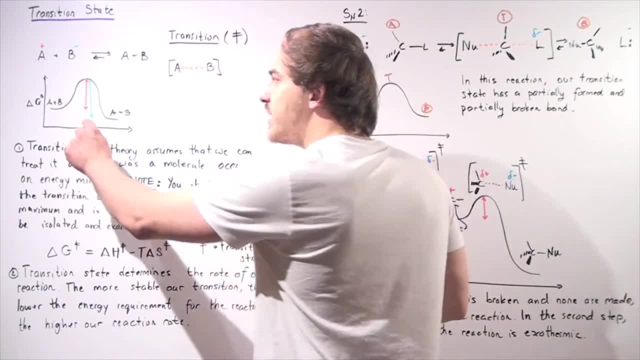 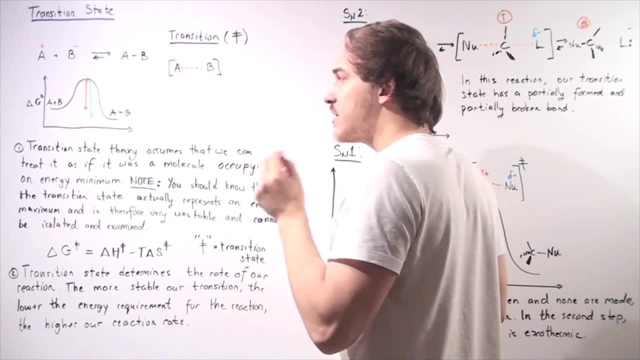 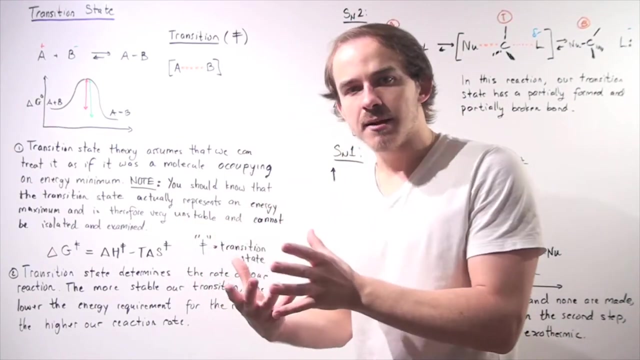 state is non-negative. It's an energy minimum. Notice that our reactants and products are found lower than our- lower on the energy level than our transition state, And that means both our reactants and products are found on the energy minimum And that means we can take them, put them in a bottle, isolate them and study. 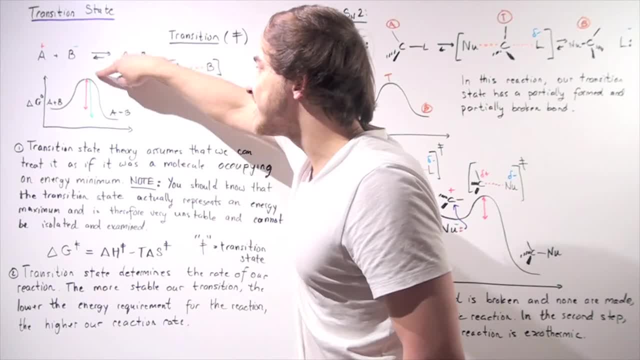 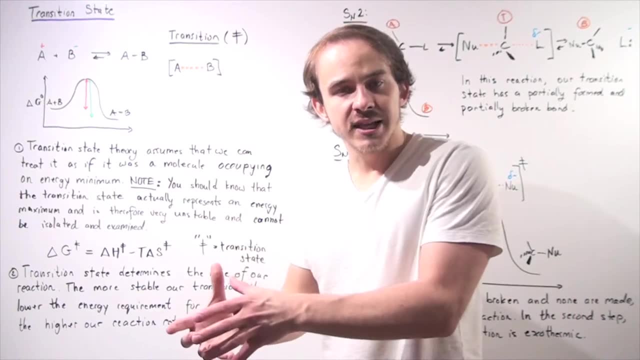 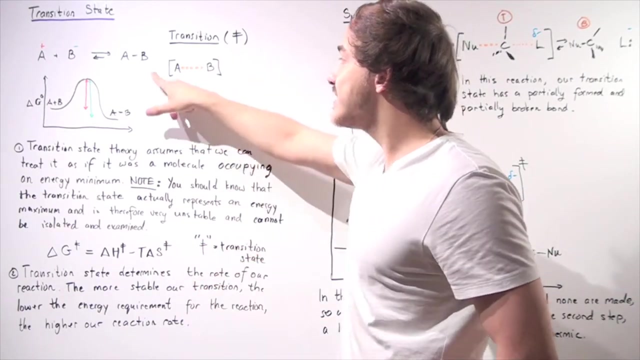 them. On the other hand, because this exists on an energy maximum, it's very unstable and there's no way that we can actually paint any matter on the energy minimum in such a way as to heat the shot, to demolish them or situations. There is no way that we can actually send anything. 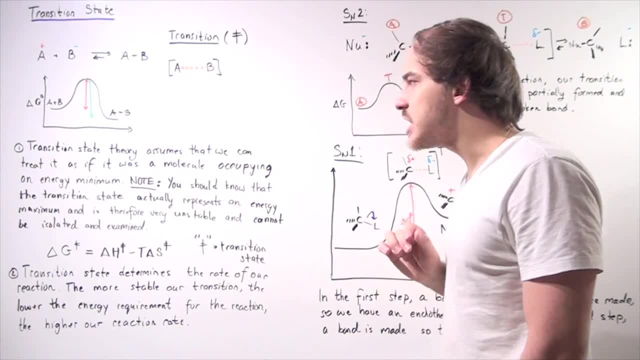 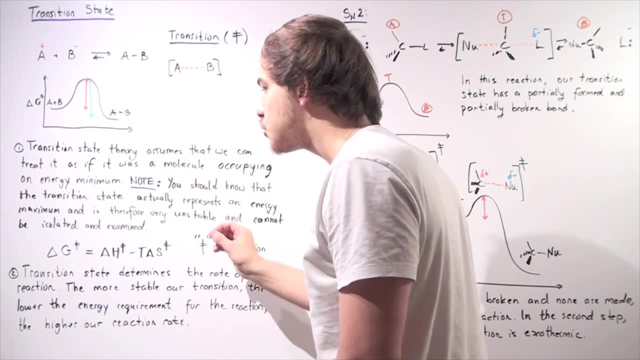 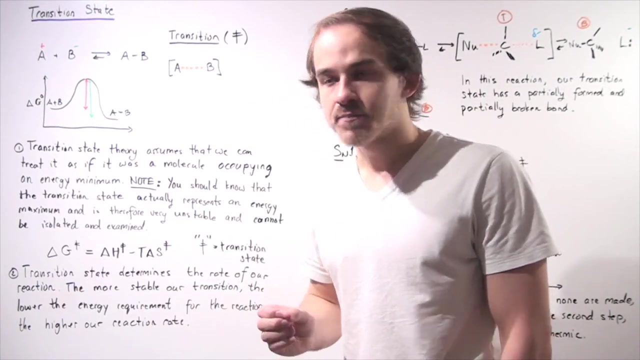 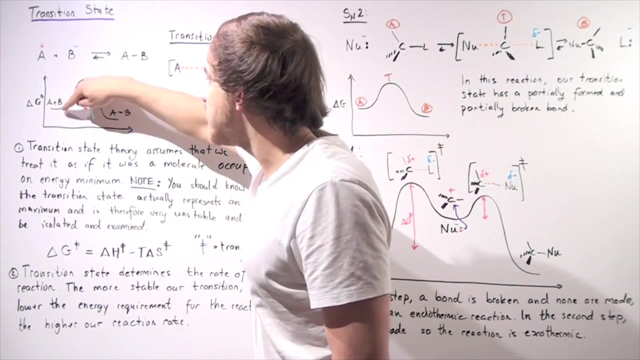 illuminated, or be пот присattan moist into thisoxygen-free solution in one shot. No way that we can V mantra to put somePaumen in the glass asf I have recently saved a throw and sit me cephal bite This activation energy. the activation energy is the energy required to surmount this energy hill and go from our initial reactants to final products. 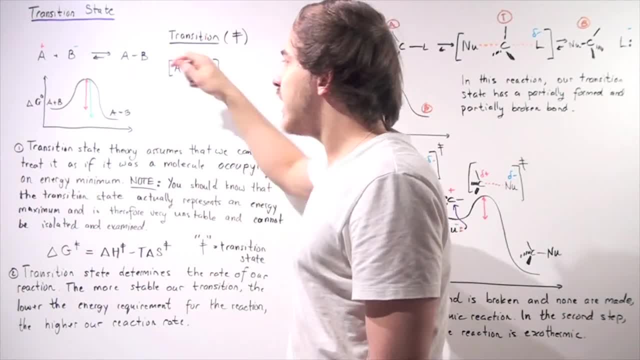 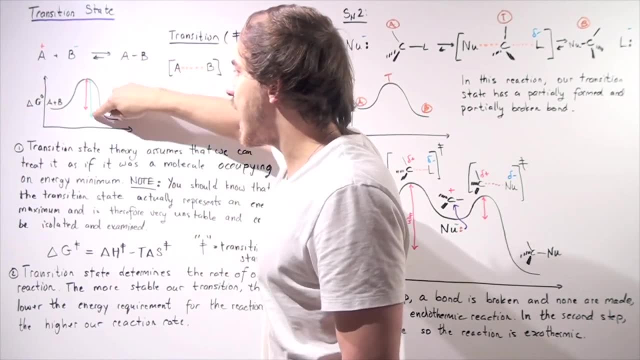 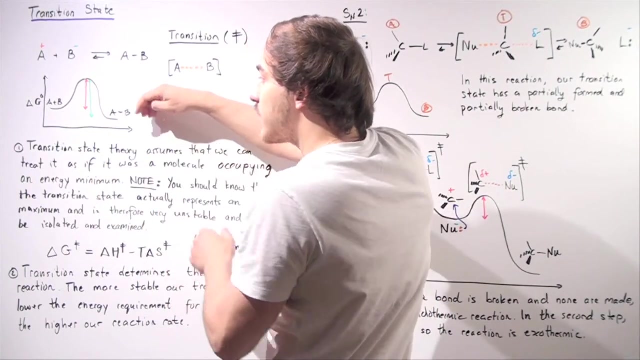 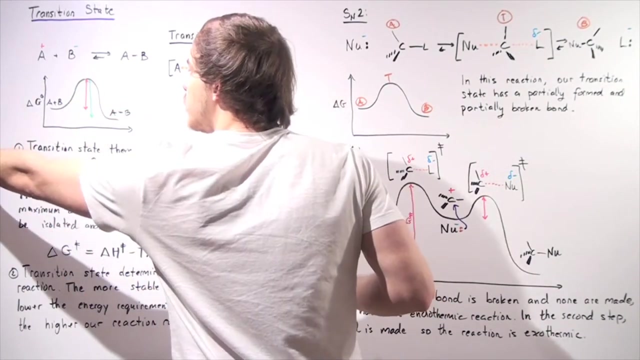 Now notice for the forward reaction we have the following red activation energy. For the reverse reaction, we have a larger activation energy And that means that our products are more stable than our reactants. Because the products are lower in energy. that means our transition state will be found higher than if we go in the forward direction. 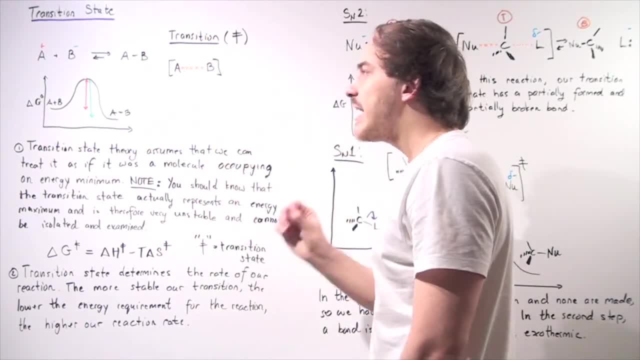 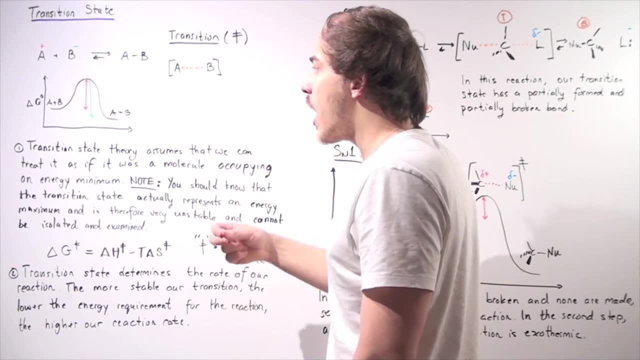 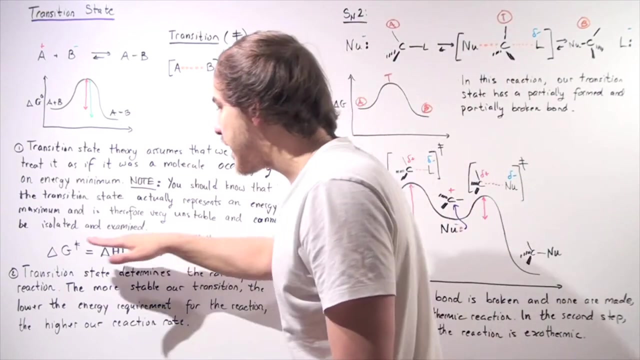 Notice that for both forward and reverse reaction, we have the same exact transition state, namely this one, but the amount of energy that is required to transverse this mountain is different. So, once again, let's go back to our change in Gibbs: free energy. 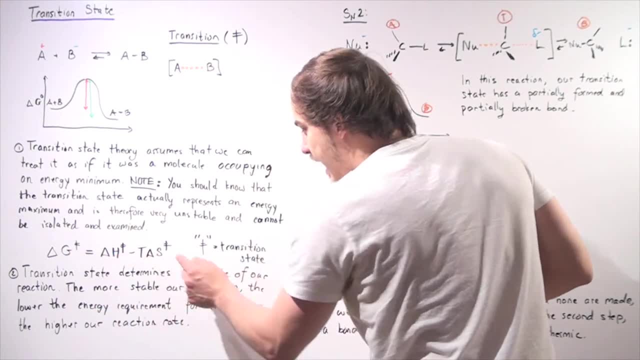 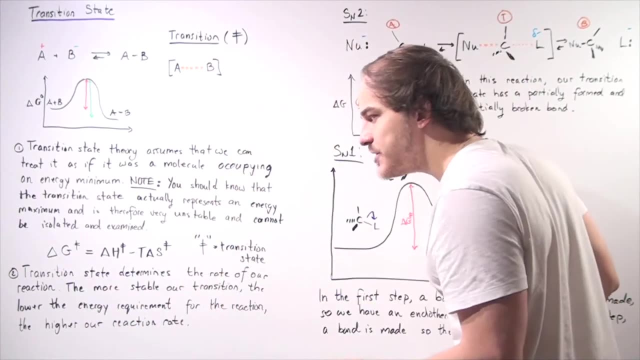 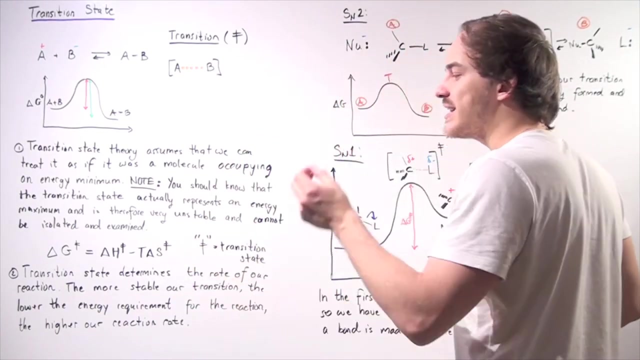 Notice that this symbol, on top of the G, the H and the S, represents the transition state. So this states that the change in Gibbs free energy of activation is equal to change in enthalpy of activation. minus temperature times. change in entropy of activation. 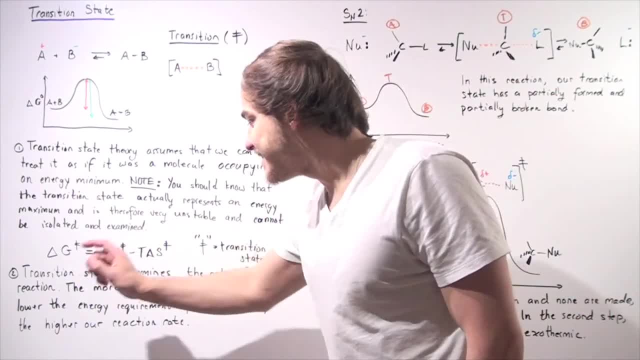 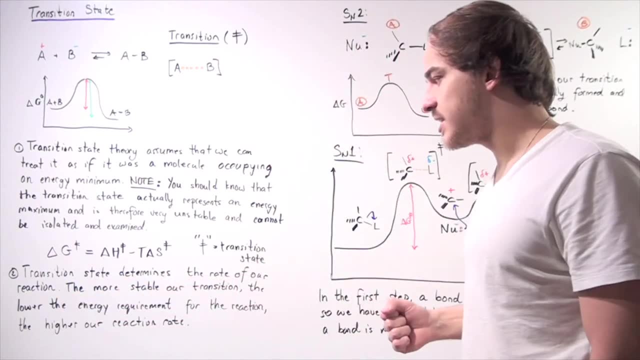 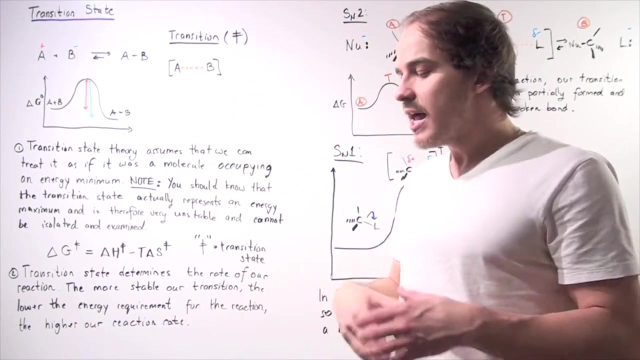 So let's go to point number two. The transition state determines the rate of our reaction. The more stable our transition state, the lower the energy requirement for the reaction. the higher our reaction rate. Now recall that thermodynamics is not the same thing as kinetics. 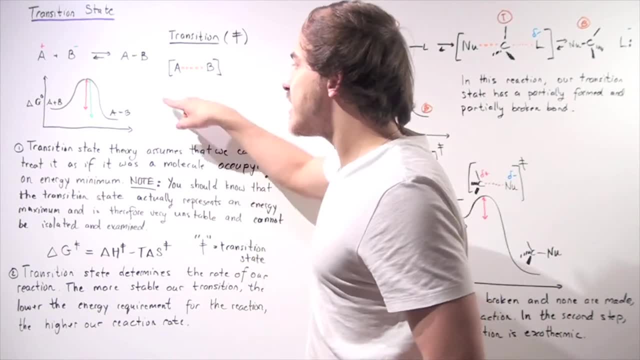 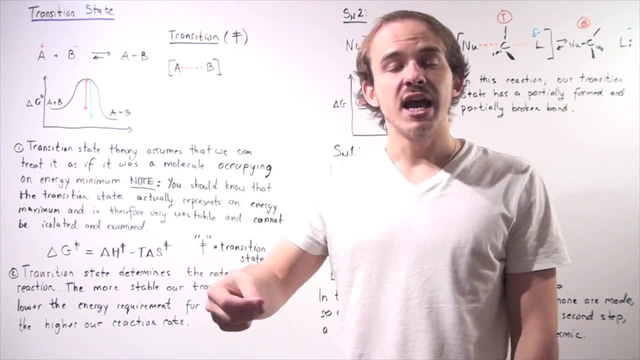 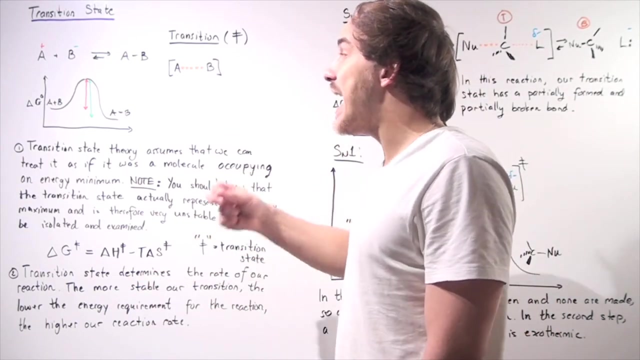 What that basically means is that the stability of our reactants and products does not actually determine the rate of our reaction, how quickly our reaction takes place. What actually determines the rate of our reaction is the level- the energy level, of our transition state. 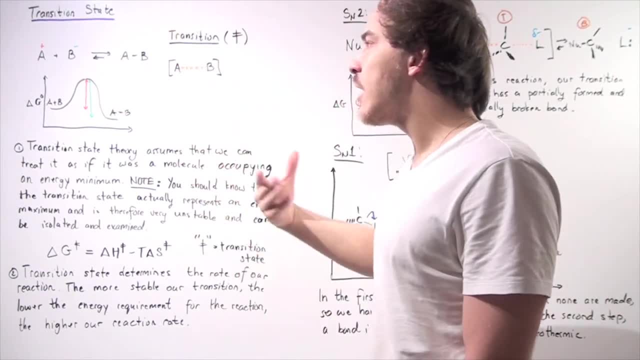 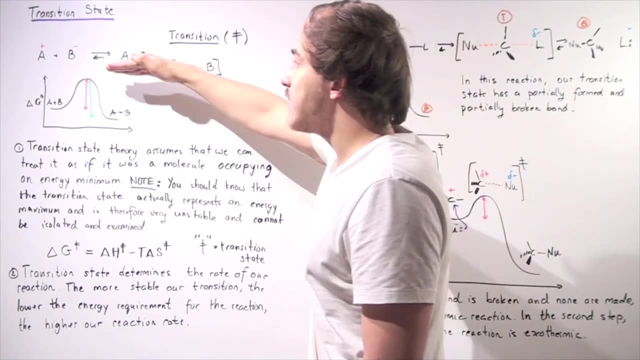 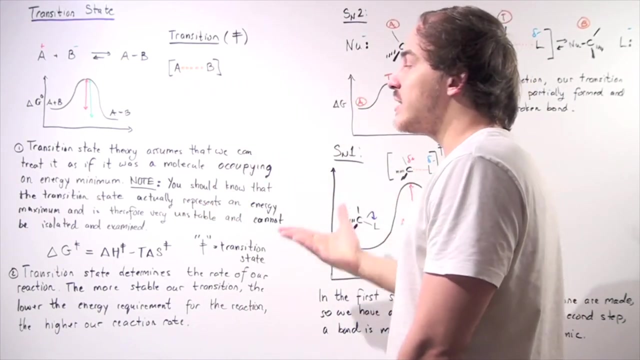 This activation energy determines how quickly our reaction will take place. If our transition state is stable, that means the energy will be lower, and so our reaction will take place quicker. If this transition state will be relatively unstable, that means we're going to have a higher activation energy, a higher barrier. 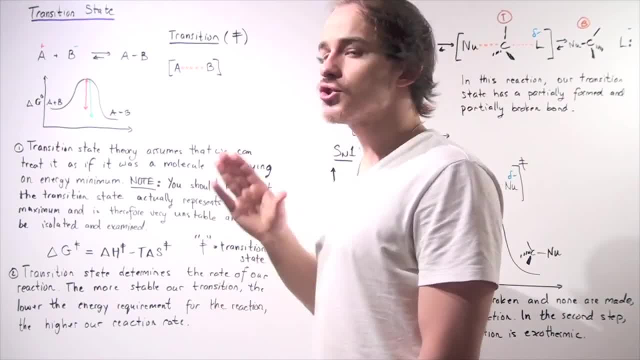 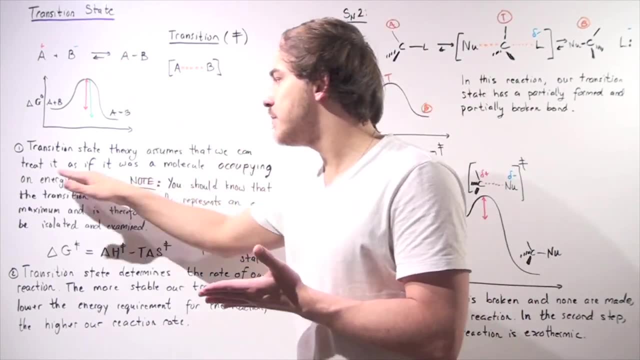 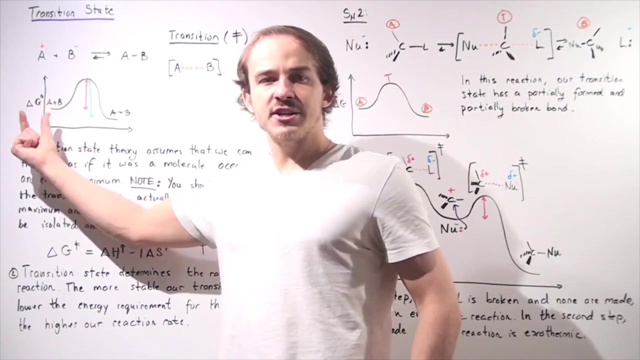 and that means our reaction will be relatively slower. So, once again, even though we can treat the transition state as if it was an energy minimum, it actually isn't. It's an energy maximum. That means it's the highest point when we go from our initial reactants to products. 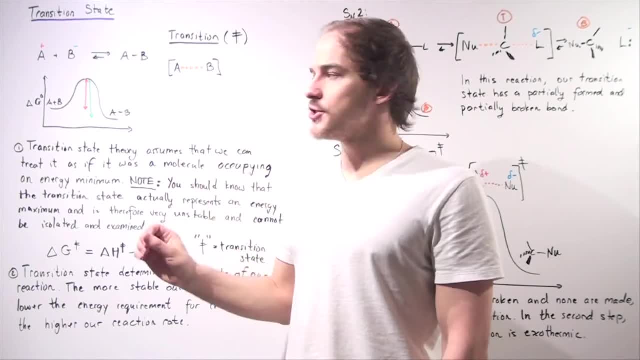 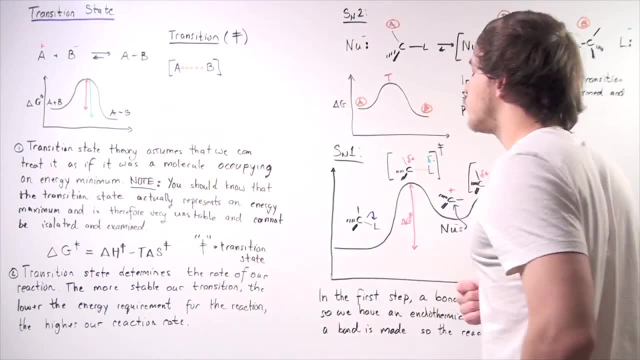 and we cannot actually isolate our transition state. We cannot put it in the bottle and study it in the same way that we can do it for the reactants and for the products. So let's examine two examples that we have studied so far. 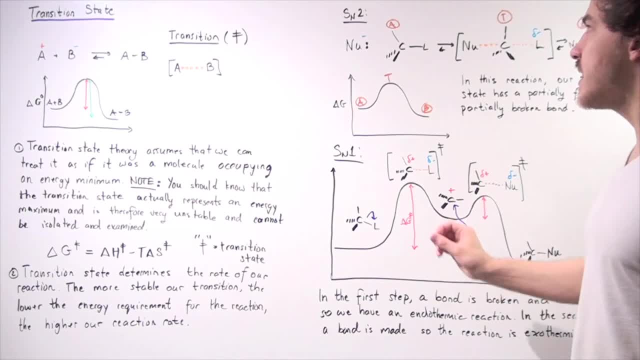 and let's examine their transition state. So let's look at a substitution nucleophilic bimolecular SN2 reaction in which we have a one-step mechanism. So in our reactant side we have the nucleophile using its pair of electrons to attack this carbon. 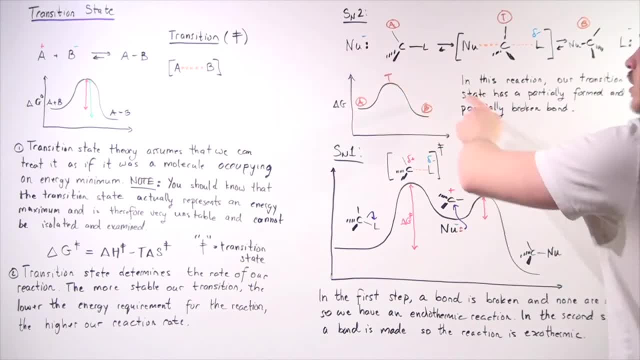 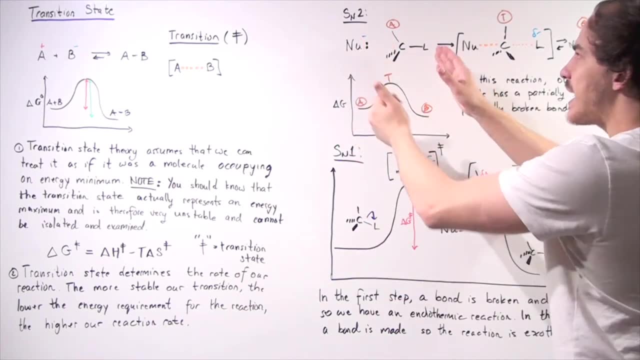 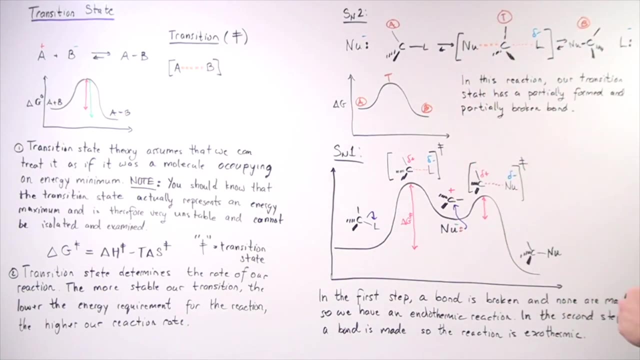 forming a bond between the nucleophile and the carbon and breaking this bond between the carbon and the leaving group, thereby kicking off the leaving group. So our initial reactants A and our final products B. Now what's actually going on in our transition state? 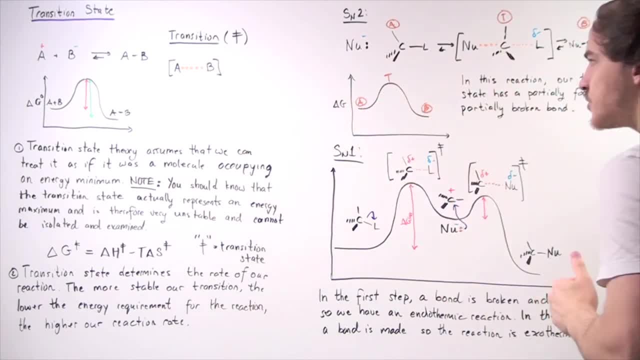 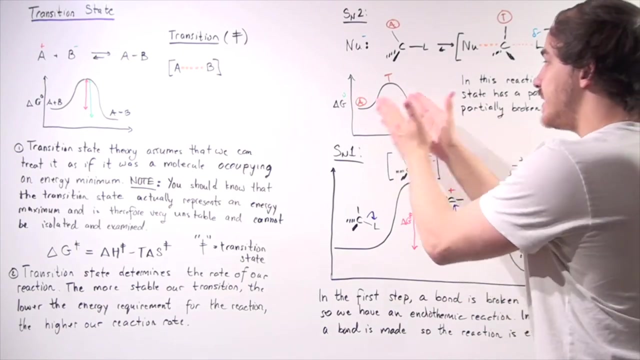 So if we look at the energy diagram for our reaction, we have the x-axis being reaction progress and the y-axis being our change. in Gibbs, free energy. Understand the state conditions. So let's put this symbol here. So notice that when we go from A to B, we have an exergonic reaction. 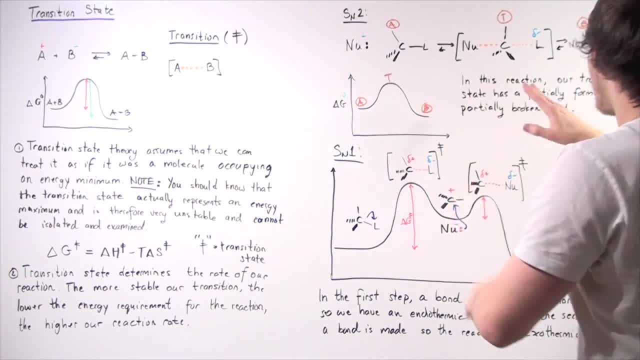 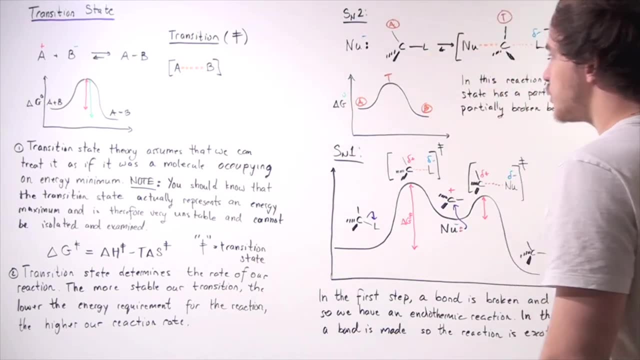 So that means our energy level is lower for our products than for our reactants. But what is actually going on in this transition state? So notice once again: transition state is the highest point on our curve. So in this reaction, our transition state has a partially formed bond. 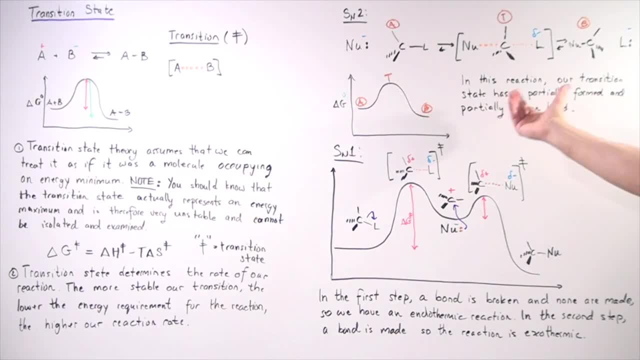 between the nucleophile and carbon and a partially broken bond between the carbon and the leaving group. And this is what it looks like. So we have the nucleophile and the carbon forming a bond and the carbon and the leaving group breaking the bond. 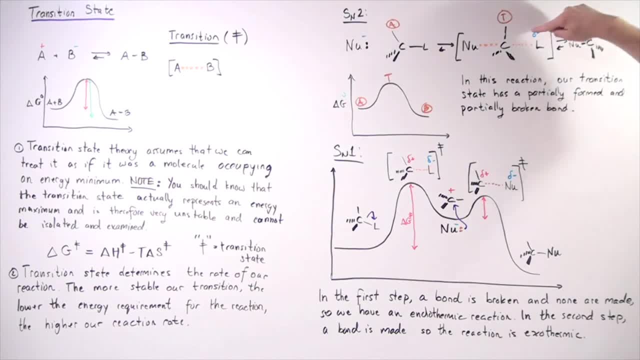 So our leaving group becomes partially negative. This carbon is sp2 hybridized and this nucleophile becomes partially positive. Now, this cannot actually be isolated. We cannot take this out and examine it individually. This is an energy maximum and that means it will not exist for a very long time. 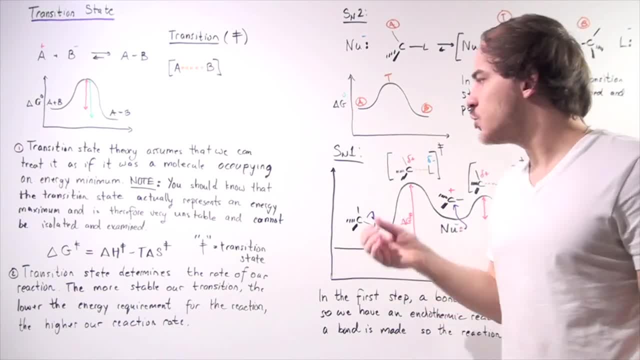 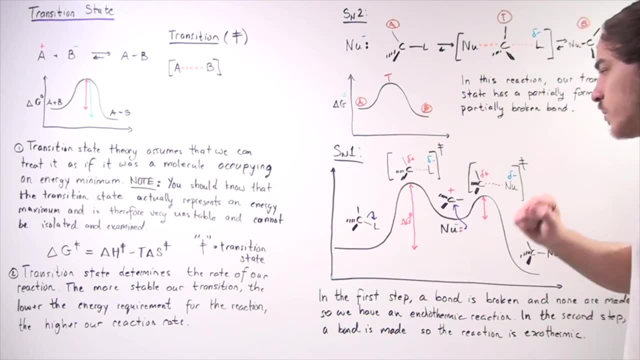 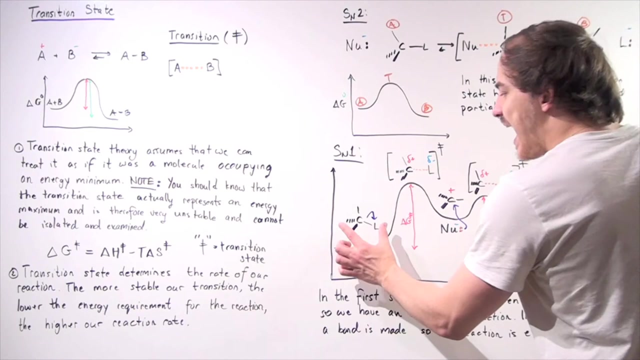 Now let's examine the SN1 reaction, the substitution nucleophilic unimolecular reaction. In this reaction we have not one but two steps, and that means we will have two energy maximums. we will have two transition states. So initially our reactants in our reactants. 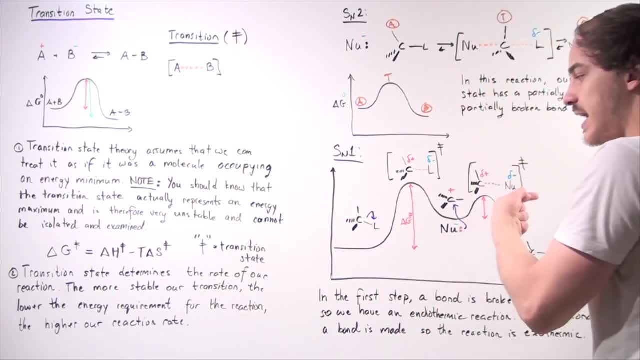 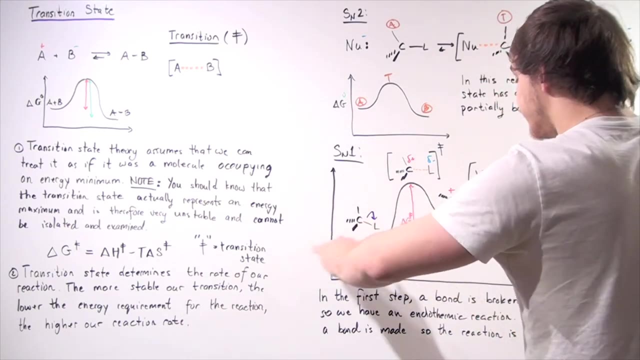 our carbon-L bond, the leaving group dissociates, This bond breaks, and so, because our bond is broken, we have an endothermic reaction. So that means our intermediate, our carbocation, will be at a higher energy level than our reactant. 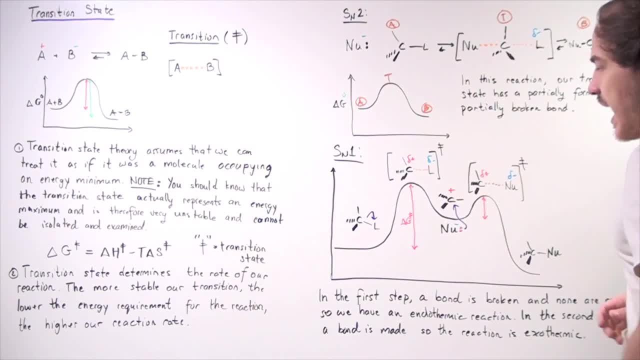 And this will be our activation energy. And if we examine our transition state, we're going to see a partially broken bond between carbon and the leaving group, And so the leaving group will have a partial negative charge. the carbon will develop a partial positive charge. 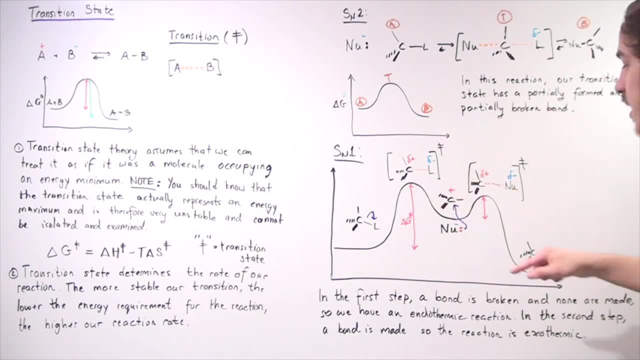 So in our intermediate step, in our second step, the nucleophile uses its lone pair of electrons to capture this carbocation attacks this carbon, And so in our transition state, we're going to have a partially formed bond between the carbon and nucleophile. 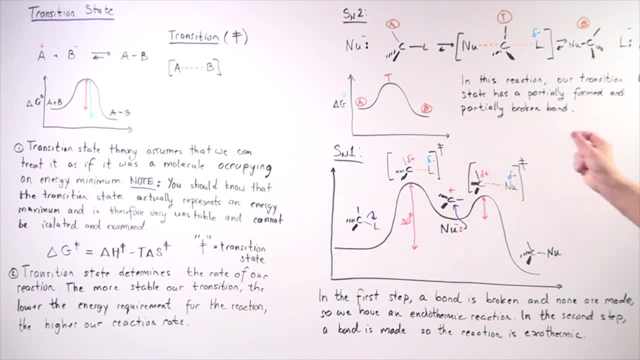 and so the nucleophile will have a partial negative charge, the carbon will have a partially positive charge, And our final product will be lower in energy than either the intermediate or the reactant. So that means our entire reaction is exergonic, And let's suppose it's also exothermic. 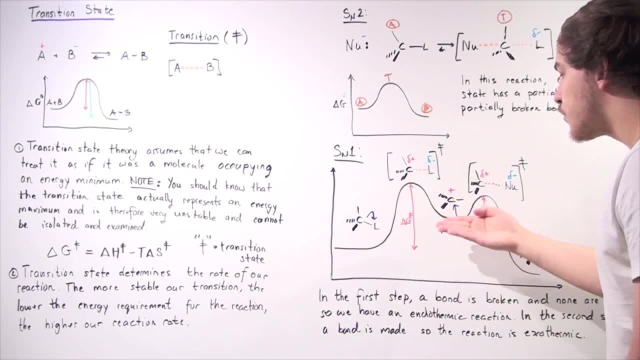 So that means, even though our first step is endothermic, our entire reaction is exothermic, And that means our products will be more stable than our reactants. So once again, in the first step, a bond is broken and none are made. 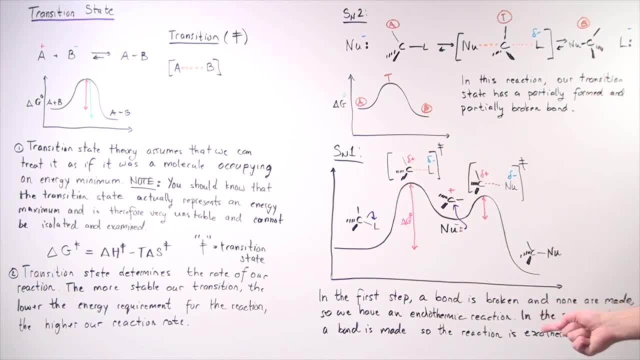 That means we have an endothermic reaction. In the second step a bond is made and so the reaction is exothermic because no bonds are broken, And altogether our entire reaction is exothermic. So once again, these are our two activation energies. 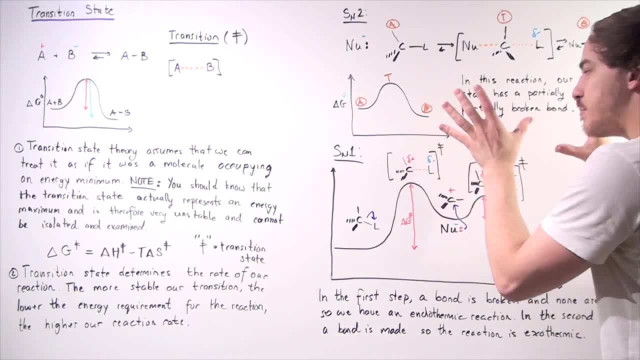 our transition states, and these are energy maxima. They cannot be isolated. So notice, we can also go in reverse, But in reverse our activation energy is different for either of these two humps. Going this way, this is our activation energy. 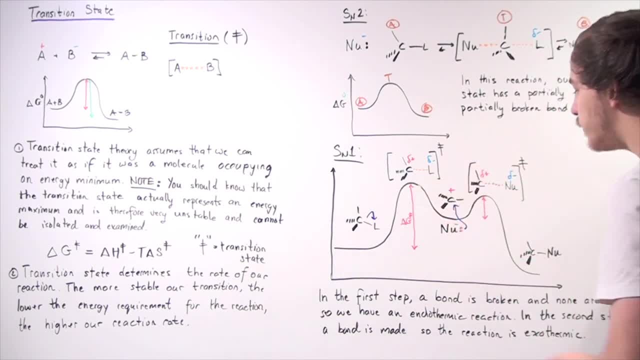 and going this way. this is our activation energy. So, going backwards, our first step is endothermic and our second step is exothermic And altogether this entire reaction is endothermic. going backwards because we go from something that is lower in energy. to something that is higher in energy.